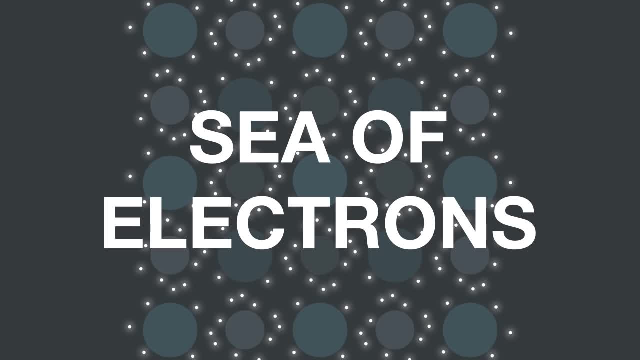 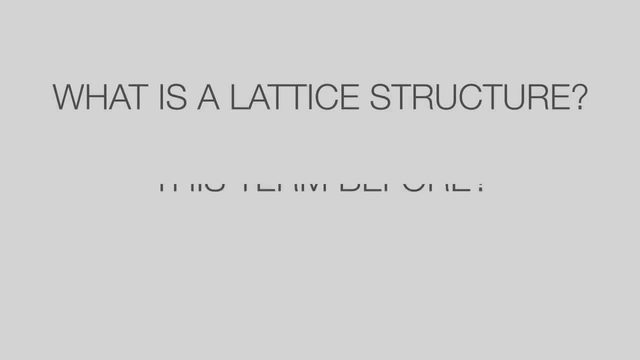 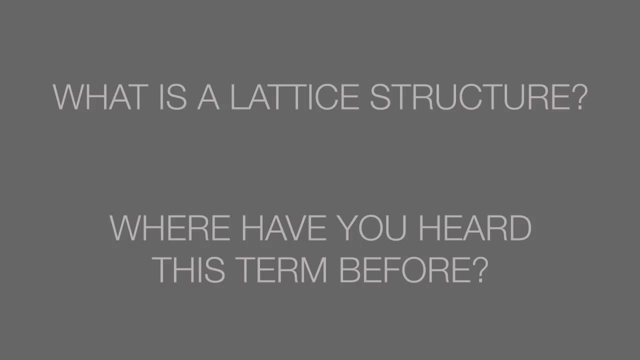 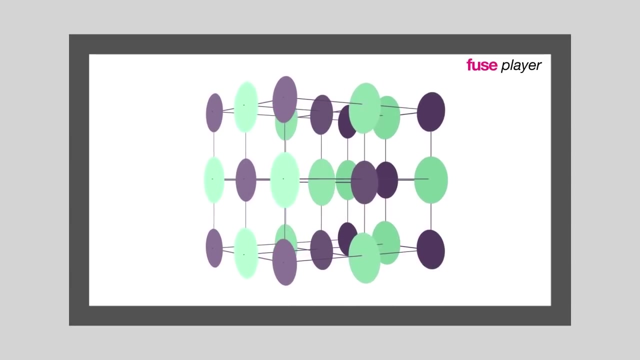 electrons are free to move around. the term sea of electrons is also used. What is a lattice structure and where have you heard this term from? Let's pause the lesson to think about this and resume when you are done. The term lattice structure means that there is a regular repeating pattern. We have heard this. 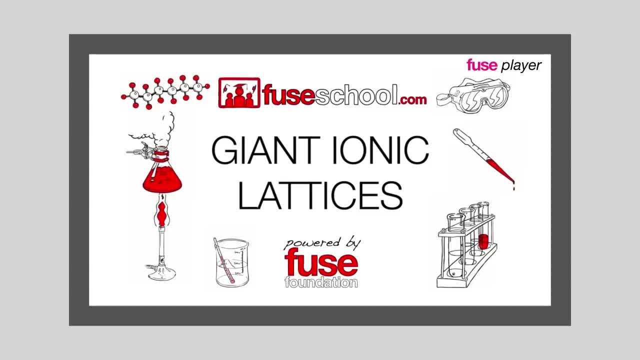 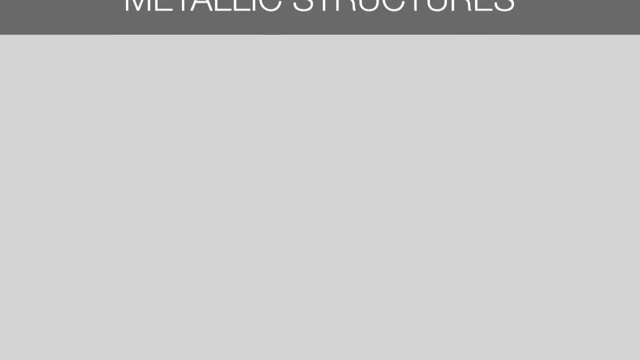 term before. when discussing ionic lattices, It is used to describe the alternating positions of the metal and non-metal ions. In metallic structures, however, there are only metal ions. These metal ions are arranged in a lattice structure, and when they are in a lattice structure, 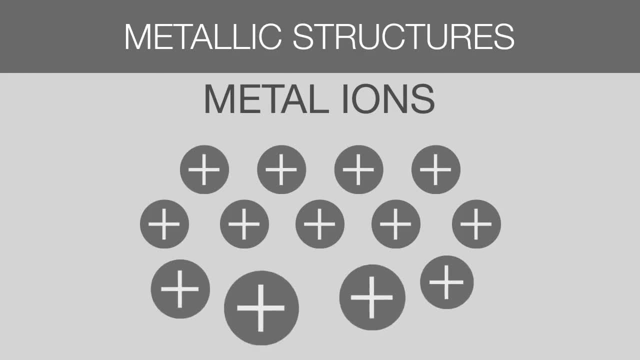 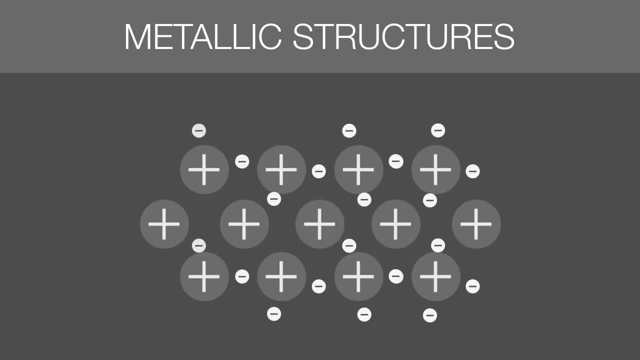 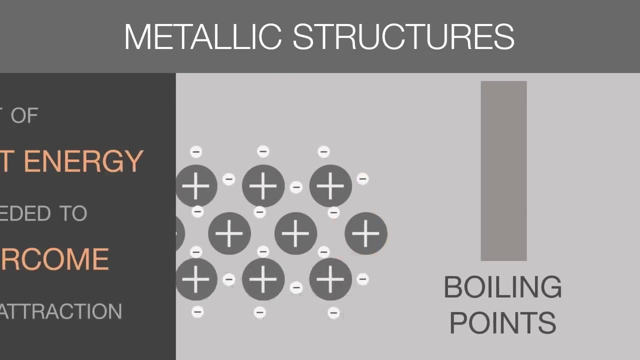 they are arranged side by side in a regular, repeating pattern. The free-floating electrons act like a glue and hold the structure in place. This is a very strong attraction and explains why metals have high melting and boiling points. A lot of heat energy is needed to overcome this. 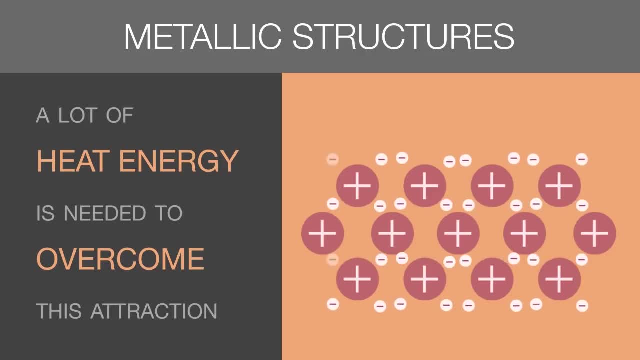 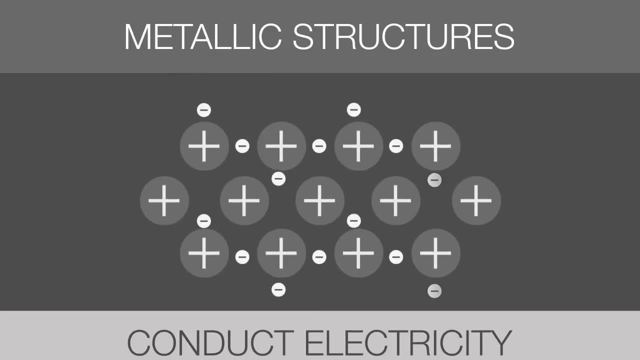 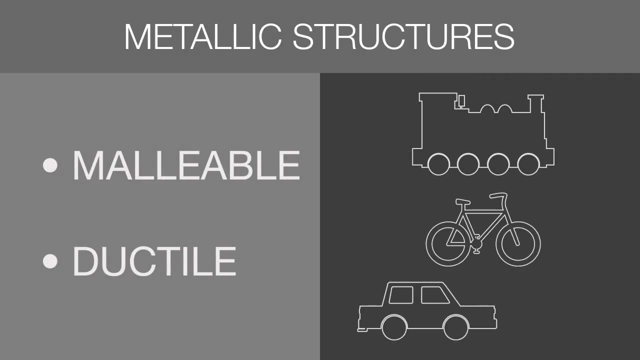 attraction. This is also why metals are very good conductors of heat. Free-floating electrons are the reason why metals can conduct electricity. Metals are malleable and ductile because no matter what shape the metal takes, the free-floating electrons will conform to that shape. The strong 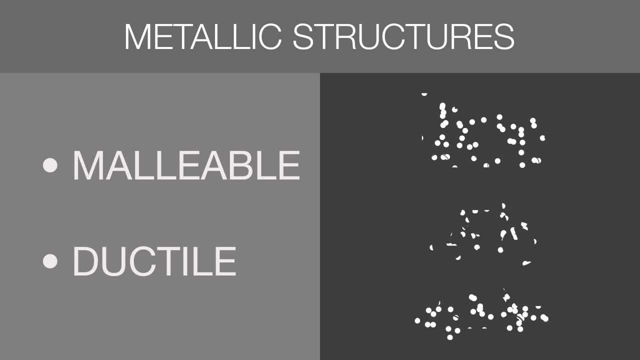 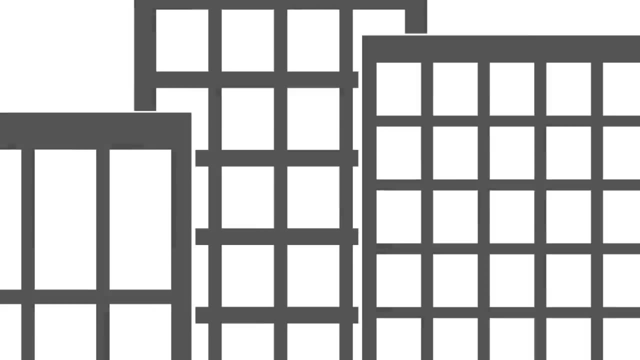 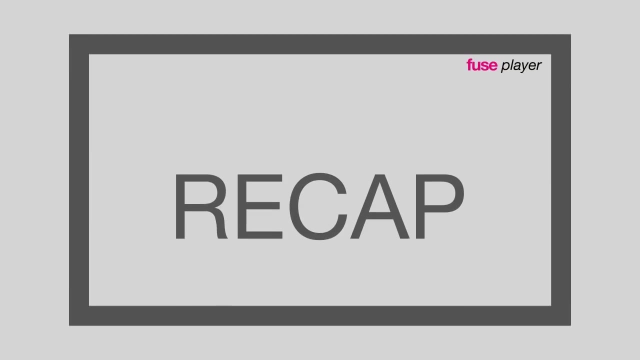 electrostatic attraction will remain and therefore the structure stays intact. Let's think about it: Cars and bicycles, trains, planes, buildings, cutlery, spectacles, furniture and endless items can be made from metals. To recap, the electrostatic attraction between metal ions arranged in a lattice structure and free-floating. 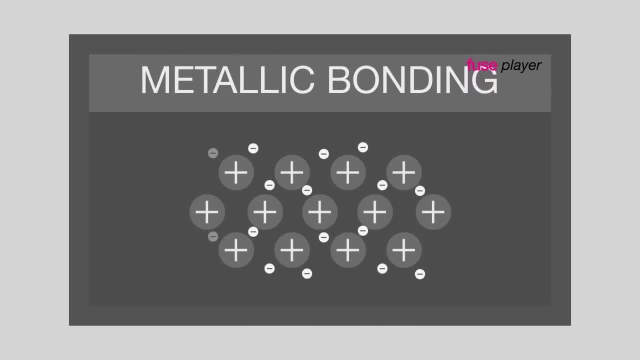 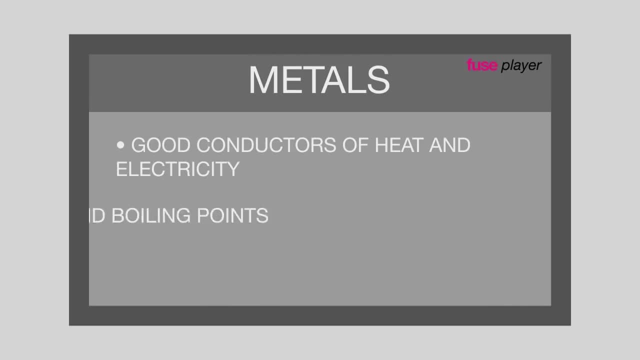 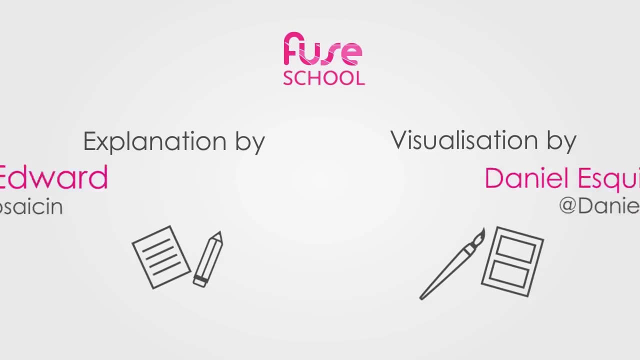 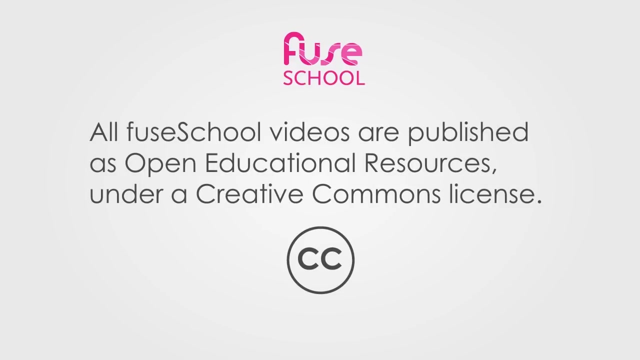 electrons is known as metallic bonding. This explains many properties of metals. They are good conductors of heat and electricity, have high melting and boiling points and are malleable and ductile. Thanks for watching.